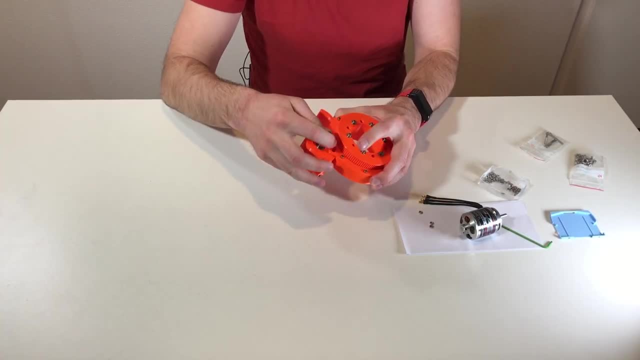 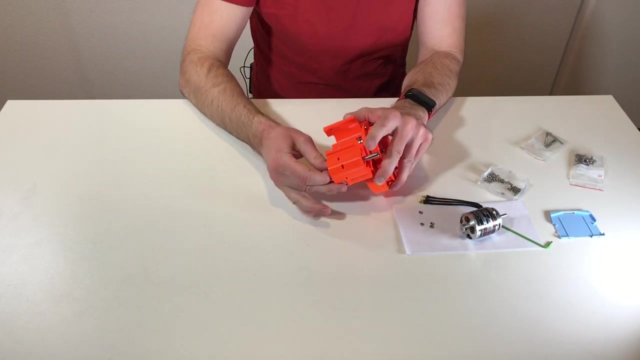 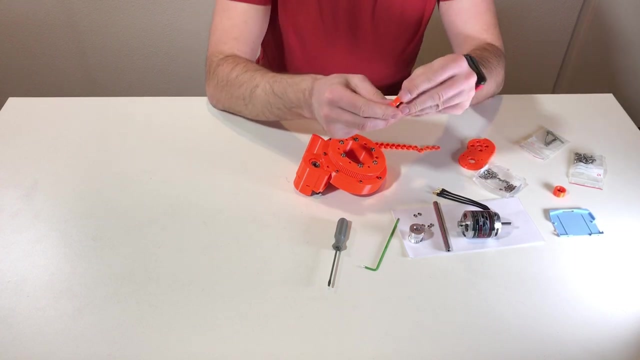 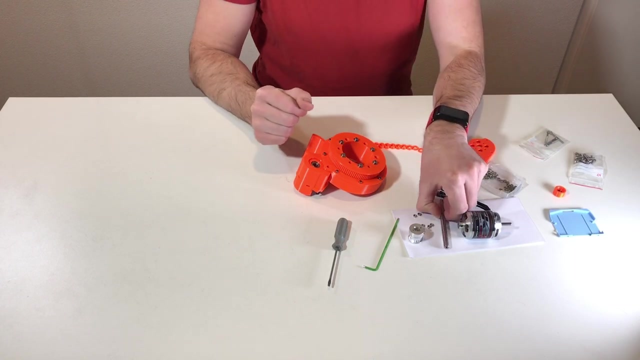 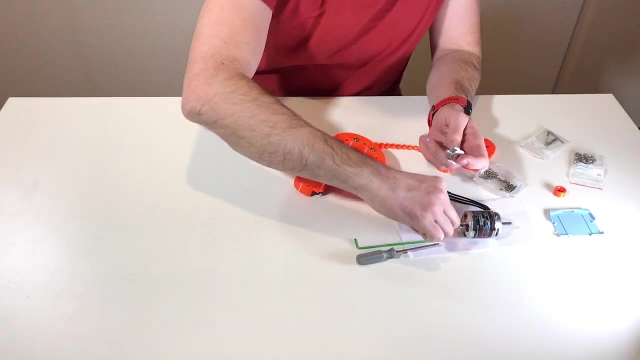 Like this, all the way in inside this bearing, like this, and I would need to install the color for the encoder over here. one more: I have some new parts, which was just ready printed. I also installed the bearing inside this holder and now let's take care of the axis. 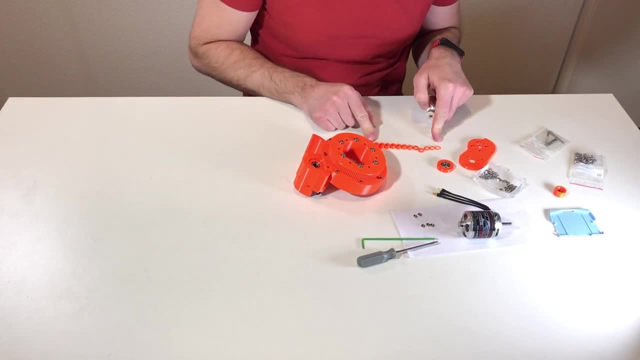 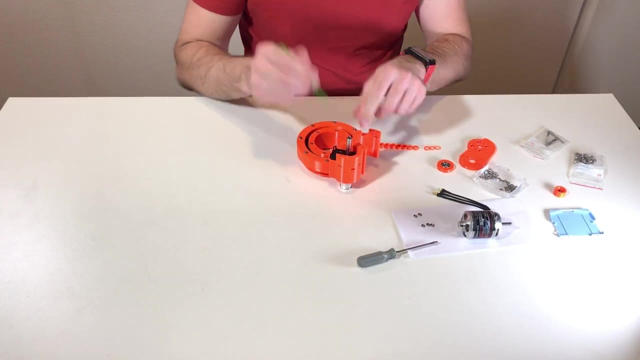 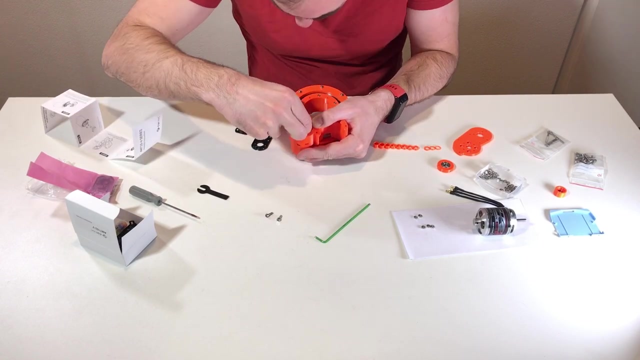 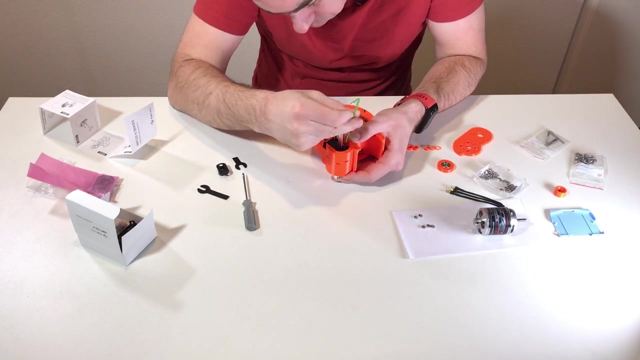 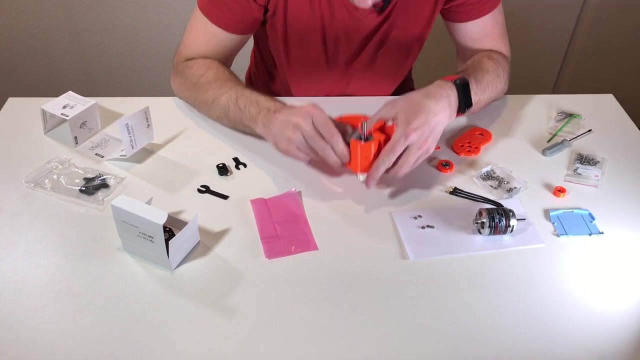 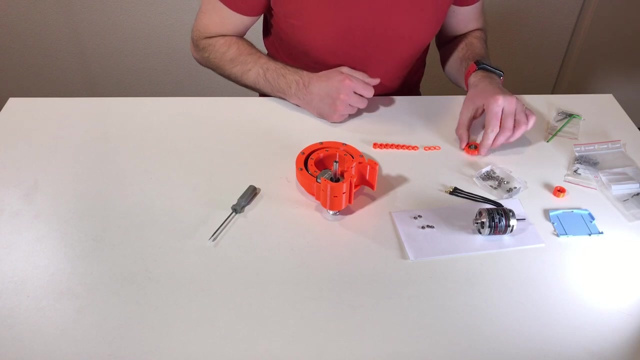 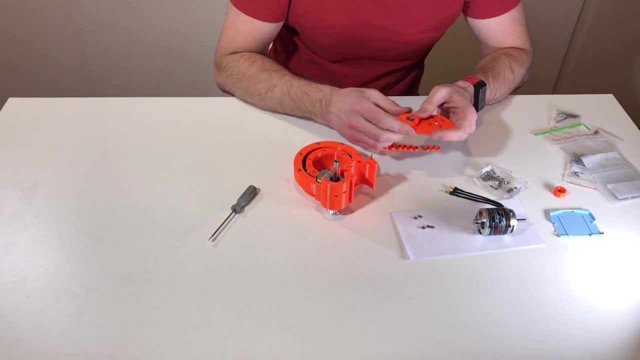 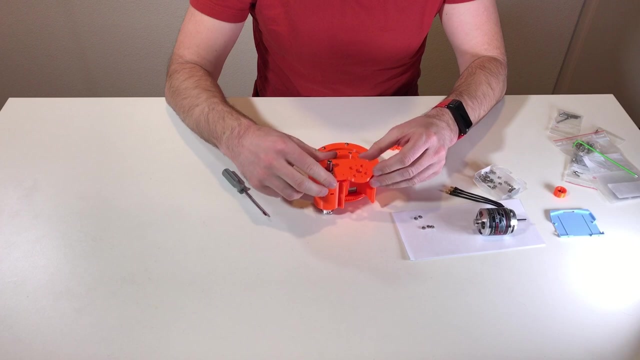 I have different spacers here. like this I can choose whatever I want. now I can install the encoder, and now the rest of the encoder. good, now the dowel pins goes here, and there is also here two placements, so let's install them. so this one goes here. 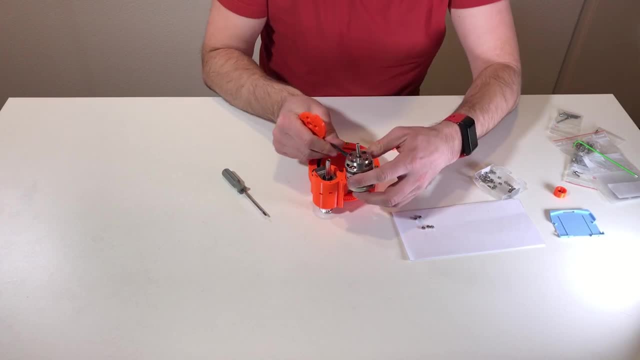 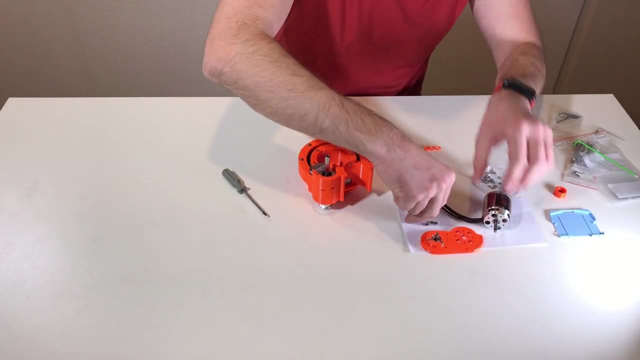 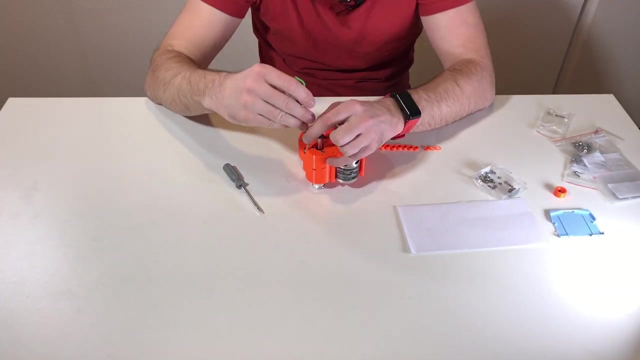 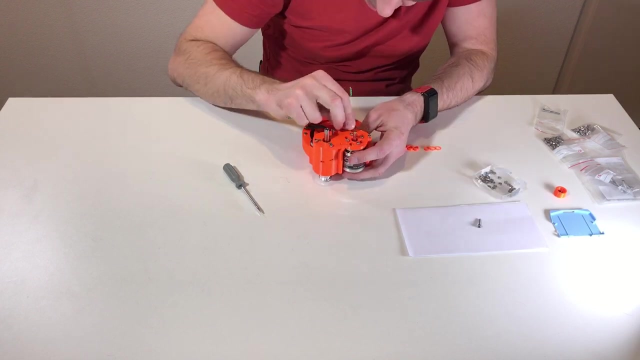 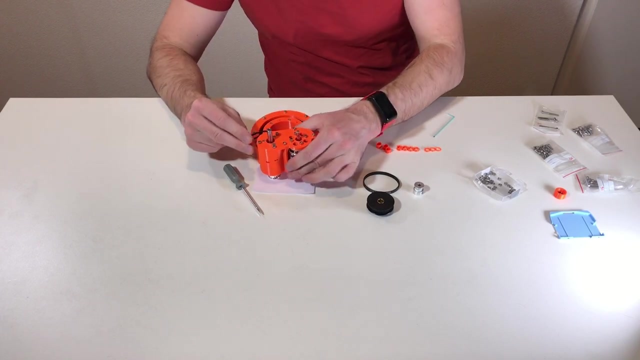 and the motor goes here. but before installing the motor, I should install the embedded nuts, in case we are going to take out so many of them, in case we are going to take out so many of them. and now the time for the pulleys and the belt. 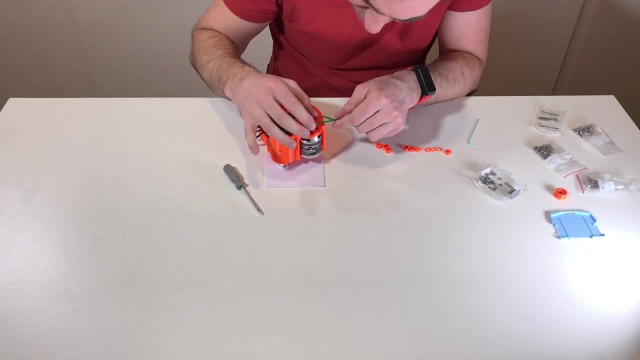 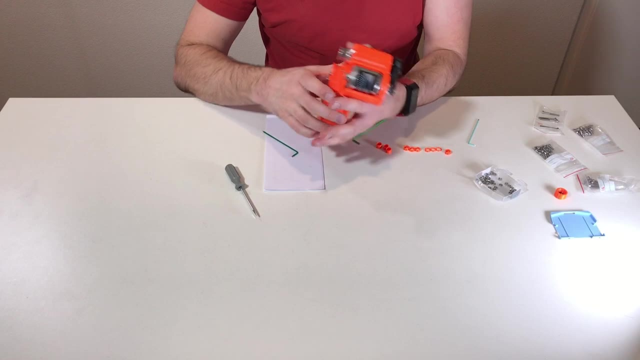 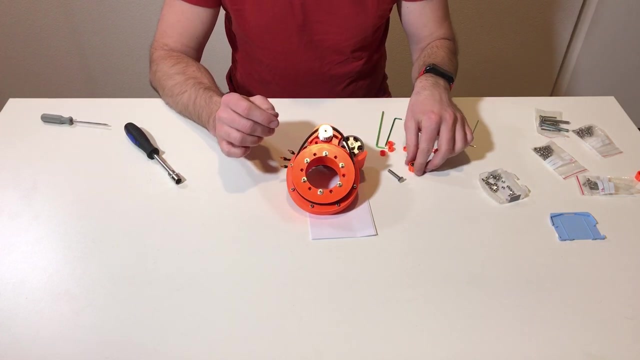 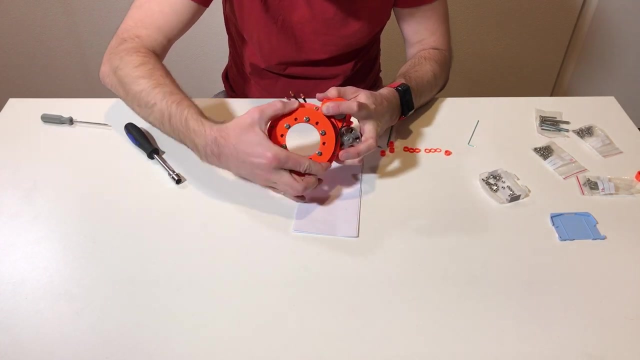 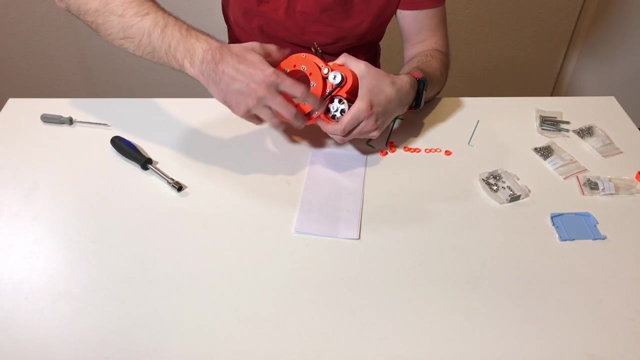 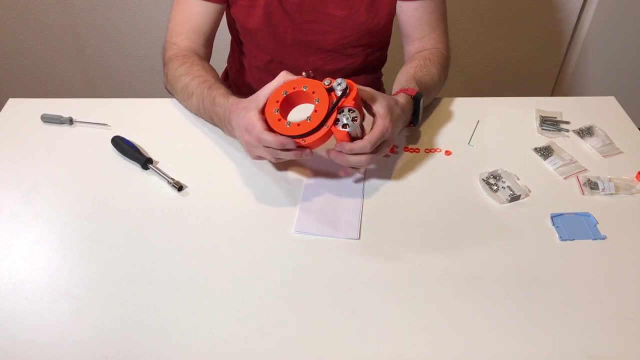 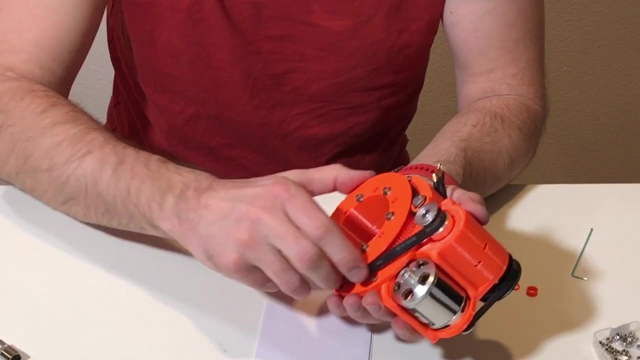 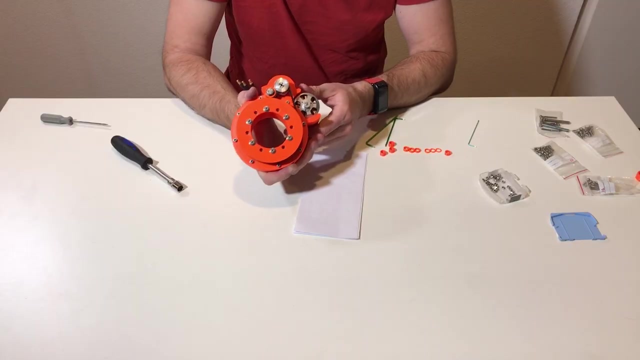 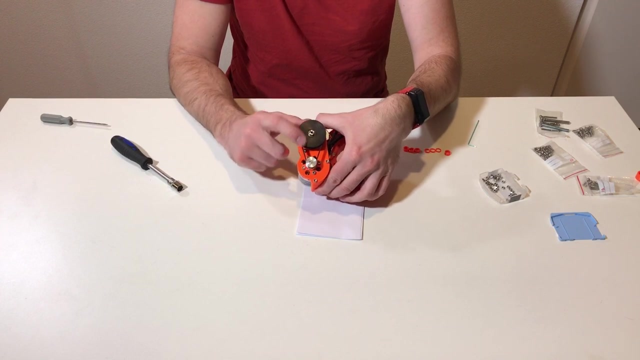 but before we need to install the spacer, Cool, and now the second belt, and over here I need to install the idler. Not bad, Nice. So the reduction ratio is 15. There is a reduction ratio of 3 here On these two pulleys And reduction ratio of 5 on these two pulleys. 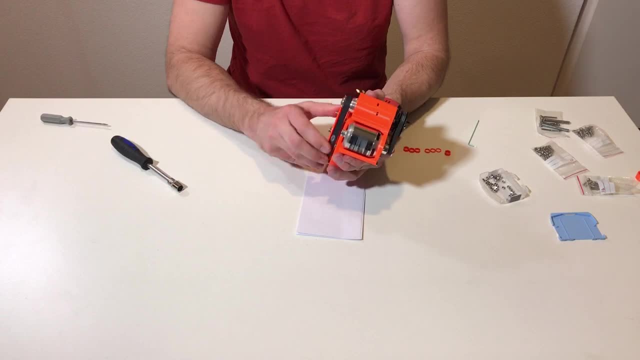 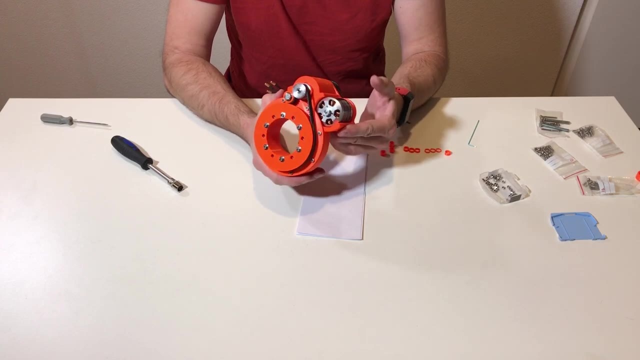 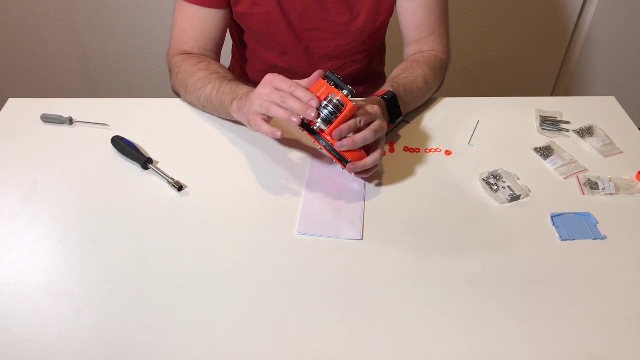 And so total is 3 times 5: 15. So, as you already Understood, This is a complete joint for the Robot arm Or for another robotic application, Whatever you want. And so it has, This motor Which has more than one Newton meter torque, And it also has an encoder. 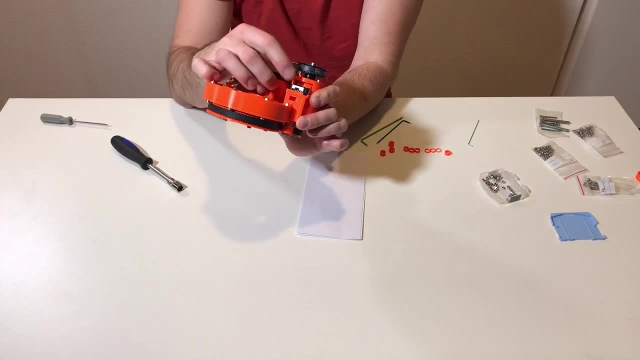 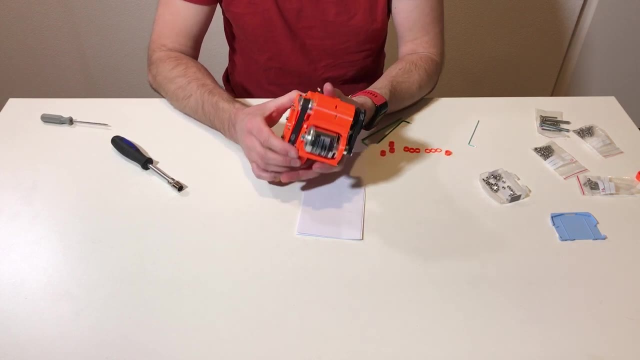 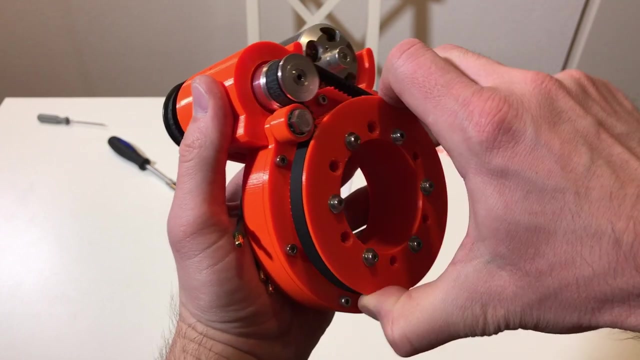 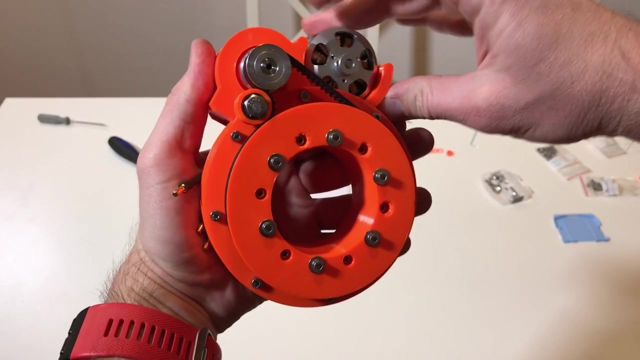 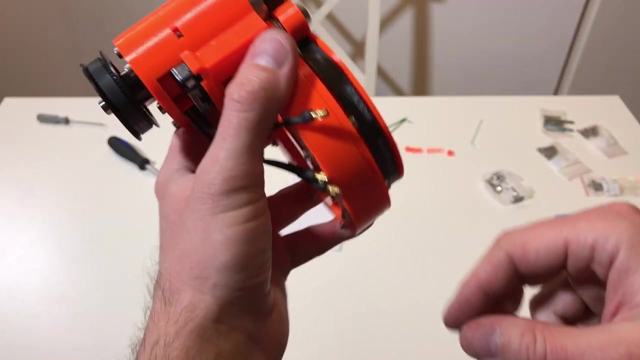 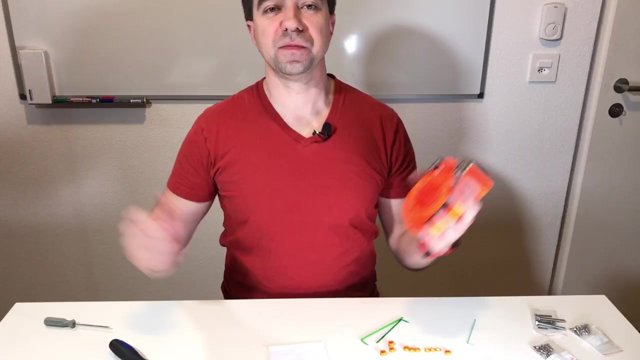 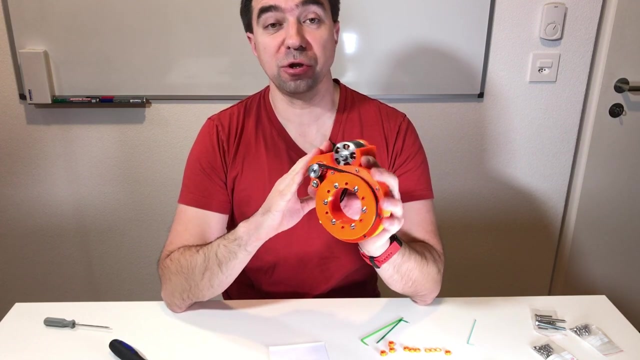 Which is just over here. So next time We're going to power it up Using odd drive controller And we'll see how it works. This is quite cool. So this is the output shaft With the same configuration. Thank you for watching this video till the end. Today, we built this robotic actuator. 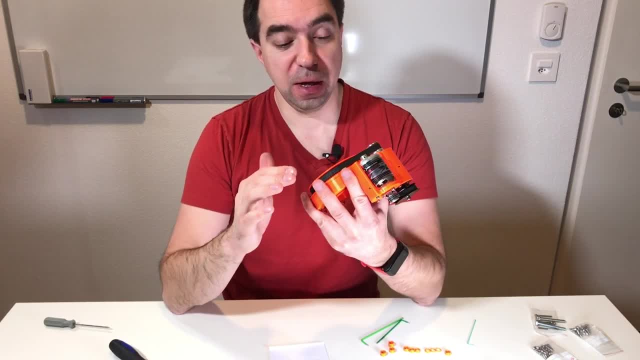 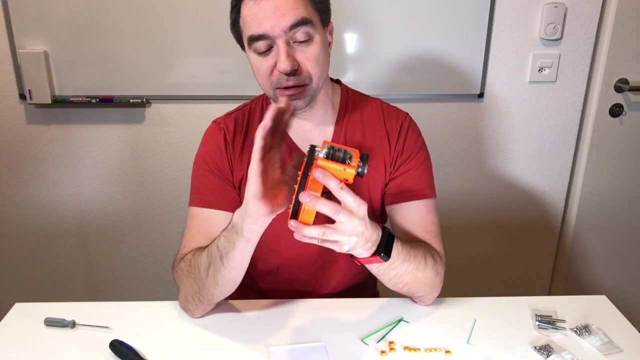 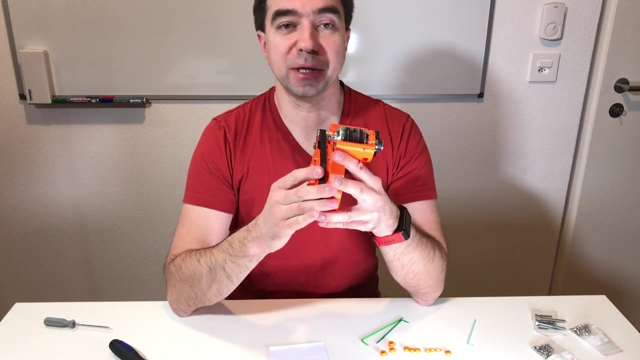 Actually it's a complete robotic joint. It has a bearing inside And also it has the motor and all reduction stages. So basically it's ready to be used. You can just Mount robotic arm here And connect all the electronics. If you're new to my channel, please consider to subscribe to my channel.